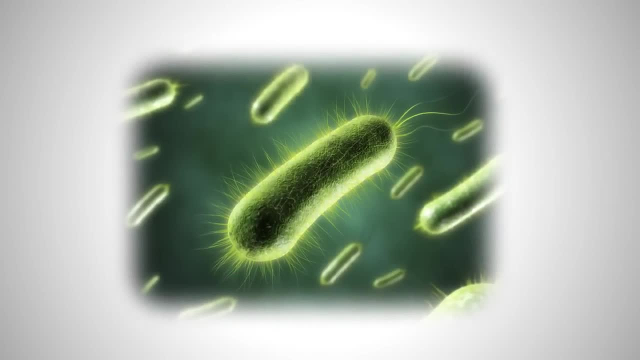 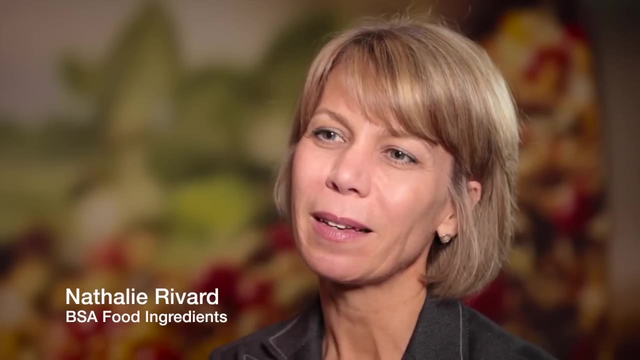 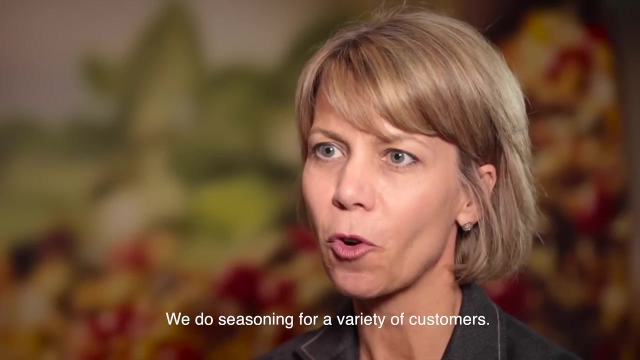 colour and low microbial count, which means the spice is safe for consumption. My name is Nathalie Rivard. I'm with BSA. BSA was founded by Marcel Barry 25 years ago. We do seasoning for a variety of different customers. 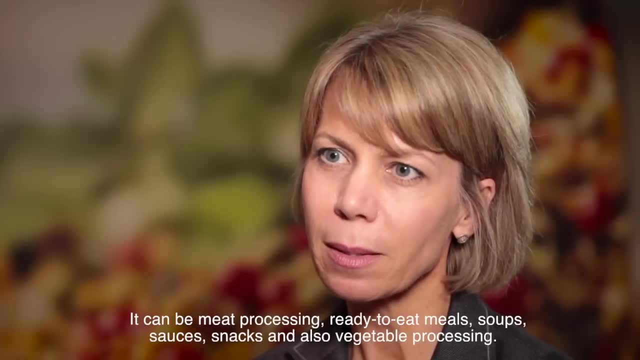 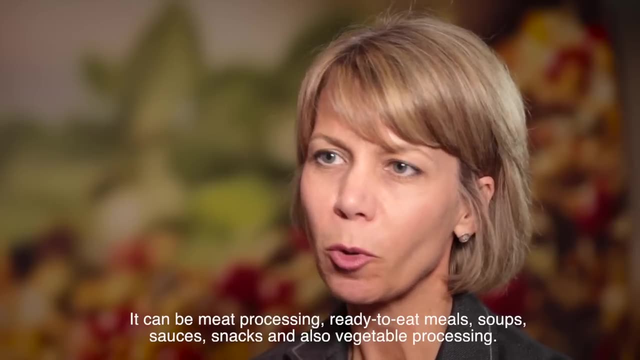 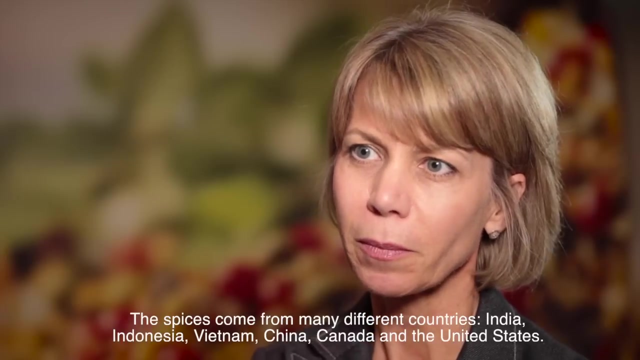 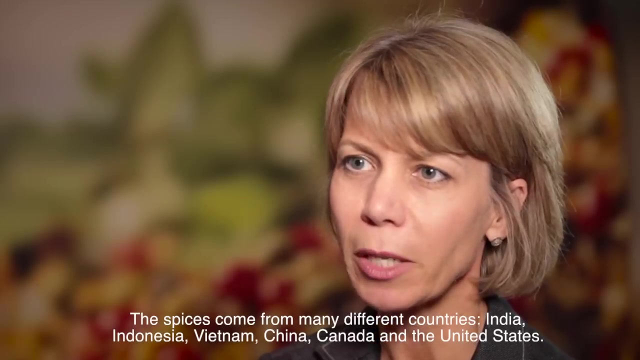 It can be meat processing, ready-to-eat meals, soup, sauce, snack and also vegetable processors. The quality of our products are very important. The spices come from many different countries: India, Indonesia and Australia, Indonesia, Vietnam, China and Canada and the United States. 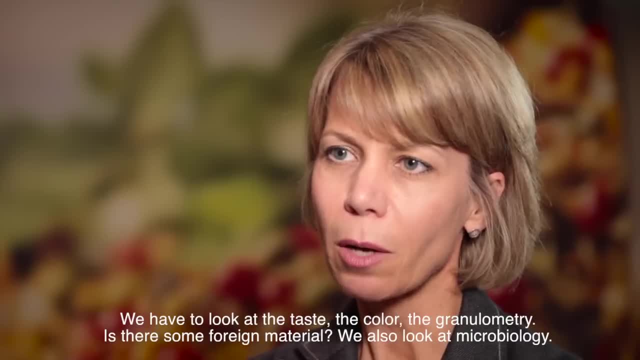 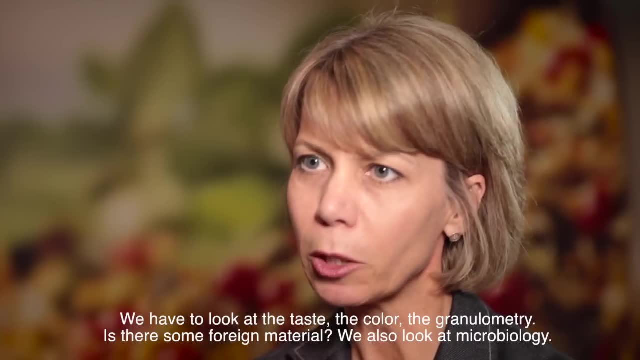 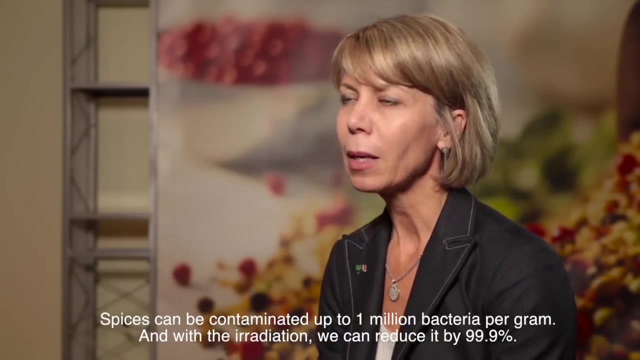 We have to look at the taste, the colour, the granulometry. Is there some foreign material? And also we look at the microbiology. Spices can be contaminated up to one million bacteria per gram And with the irradiation it can reduce by 99.9%. 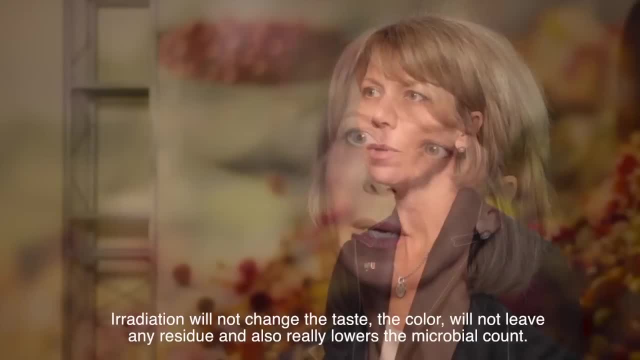 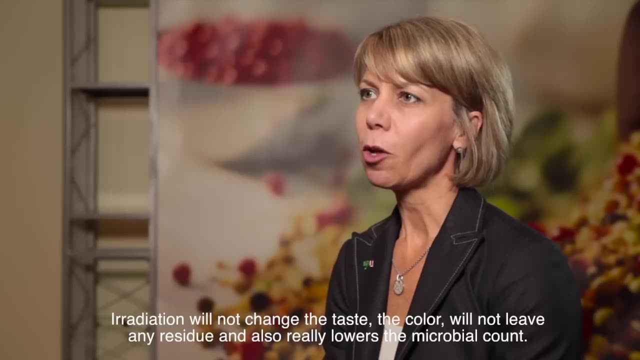 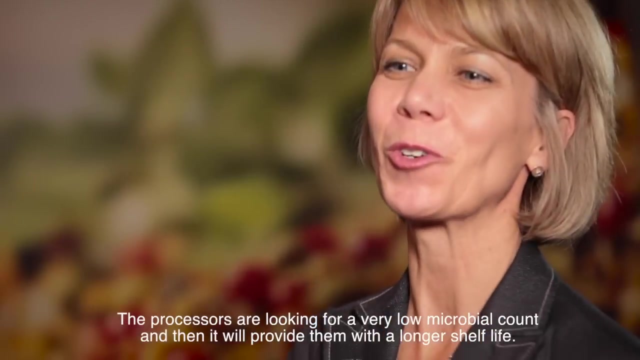 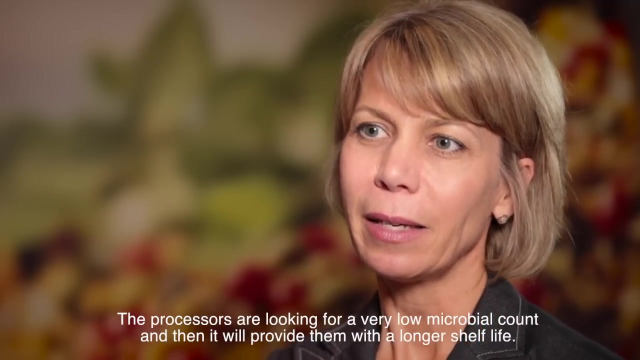 will not offer that kind of reduction. Irradiation for us will not change the taste, the colour, will not leave any residue and also is really lowering the microbiological count. The processor, you know, are looking for a very low microbiological count and then it will provide them a longer shelf life. The 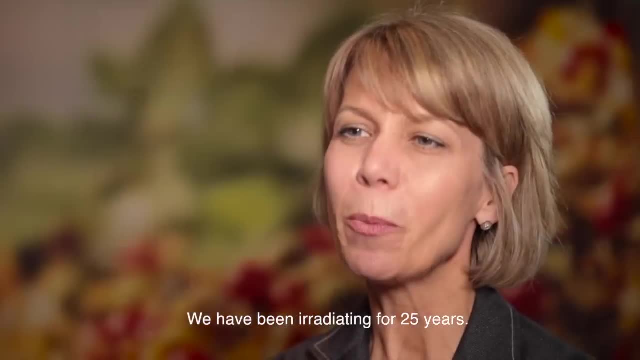 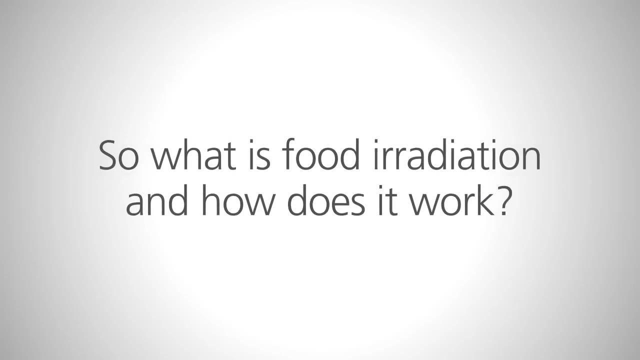 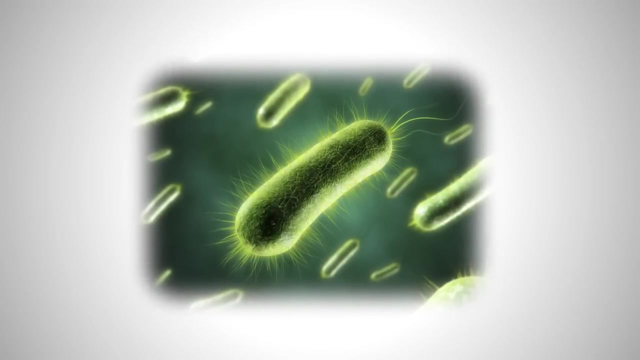 counts are lower when we use irradiation. We've been irradiated for 25 years. So what is food irradiation and how does it work? Meat, poultry and spices, for example, have a variety of microorganisms on them that can make people sick. These 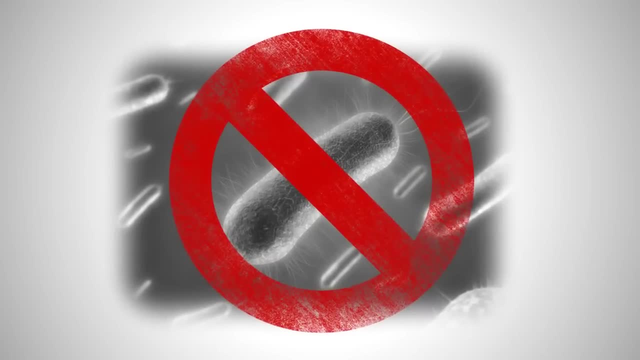 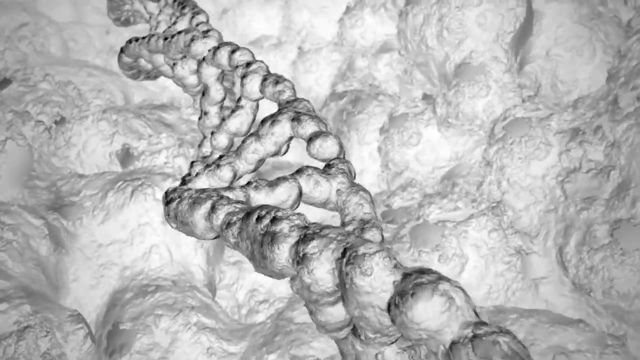 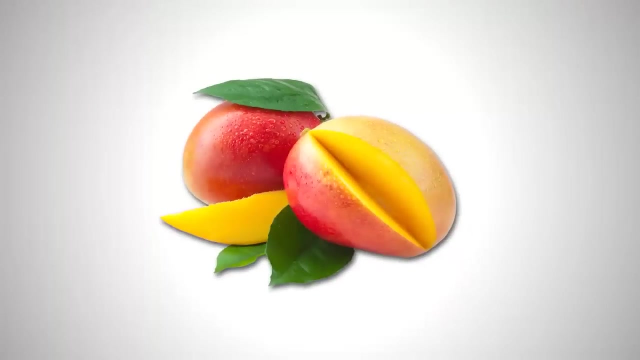 need to be controlled to avoid causing harm to consumers. Living things like pests and microorganisms need DNA to function. Irradiation disrupts the DNA and kills the living microorganisms. Irradiation has minimal impact on things which are not alive, such as food. 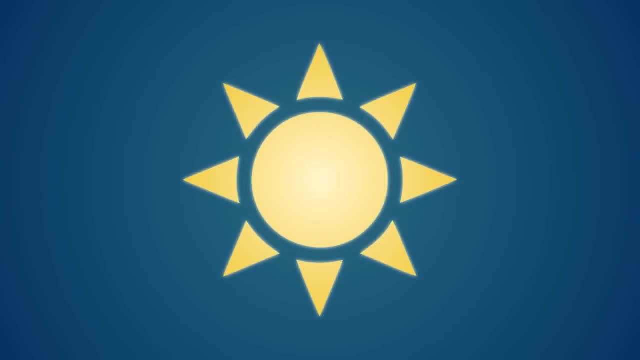 Irradiation is a process that uses energy in a form of radiation. just like radiation from the Sun, This radiation comes from man-made sources such as cobalt-60, electron beam or x-ray machines. Here's how this energy is put to work. A box of spices, for example, arrives at an. 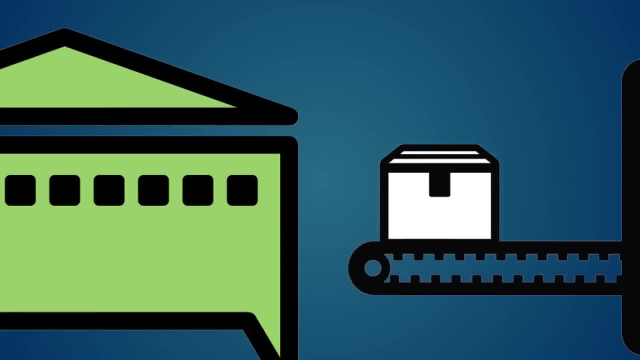 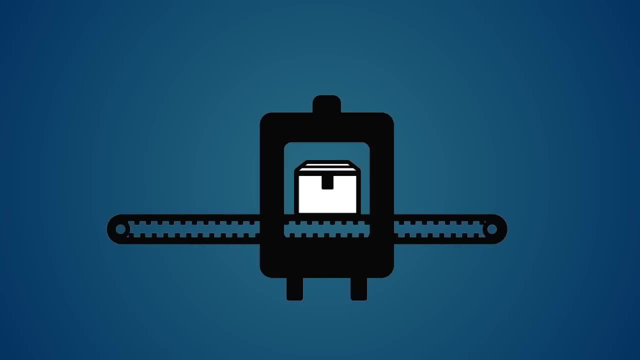 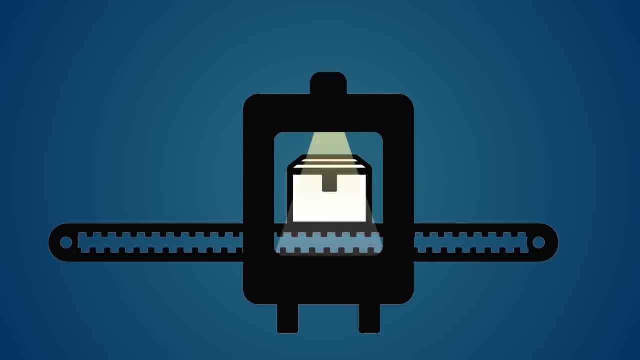 irradiation facility. It's loaded onto a conveyor. The conveyor moves the box into the irradiation chamber and past the source of radiation, The box spends a designated amount of time exposed to the radiation. The energy travels through the box to kill microorganisms inside, Then moved out of the. 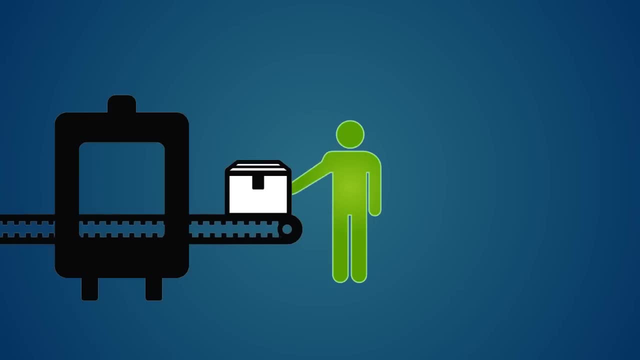 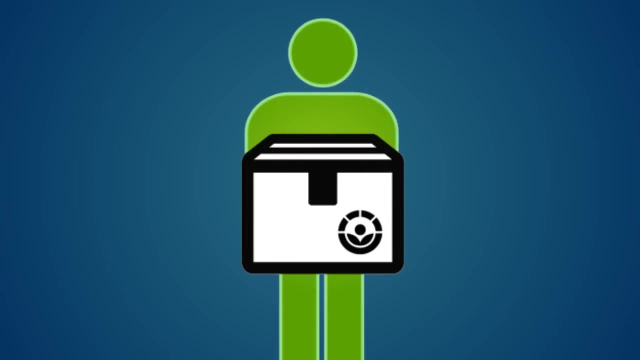 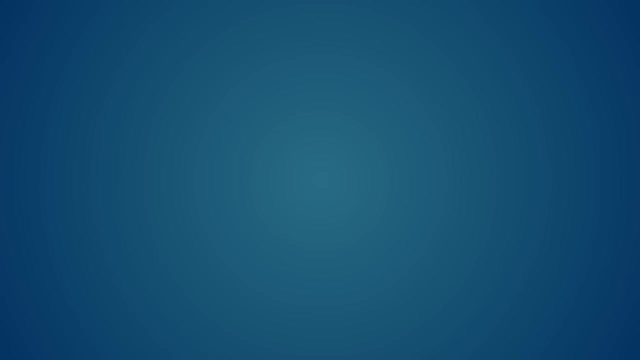 chamber. The box and its contents are safe to handle immediately and labeled with the Radura symbol, the international symbol indicating treatment by radiation. The box is loaded into a truck for delivery to grocery stores. As an example, Nordian's Gamma Centre of Excellence treats food products such as spices. 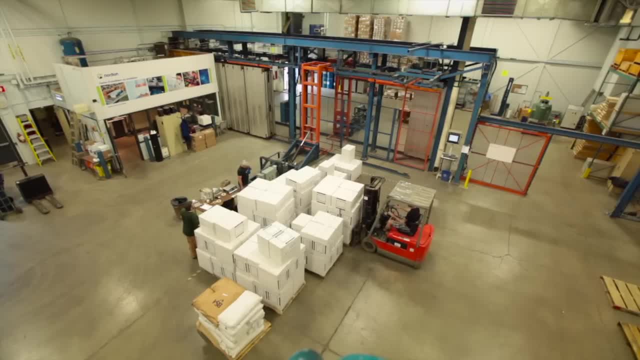 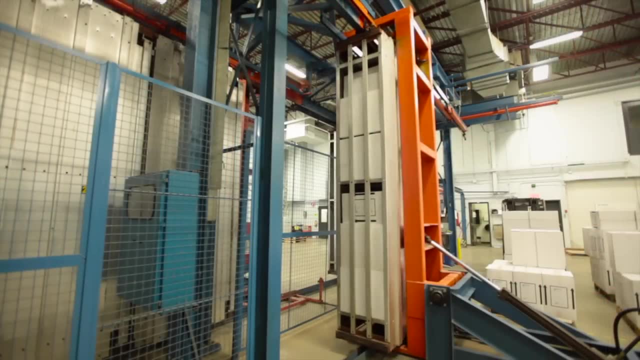 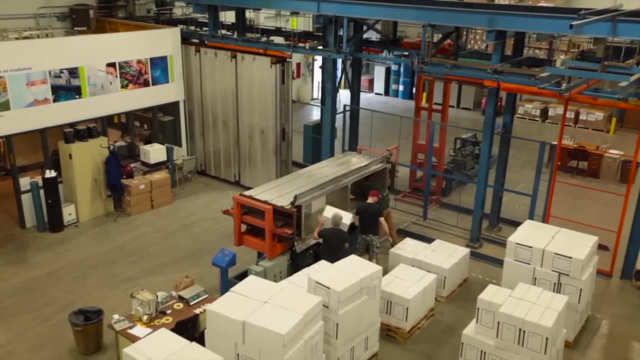 from BSA. At the facility warehouse boxes of spices are received, loaded into containers called carriers and started through the irradiation cycle. A pool of water safely captures the gamma rays from Cobalt-60 while the product is being loaded outside Inside the irradiation. 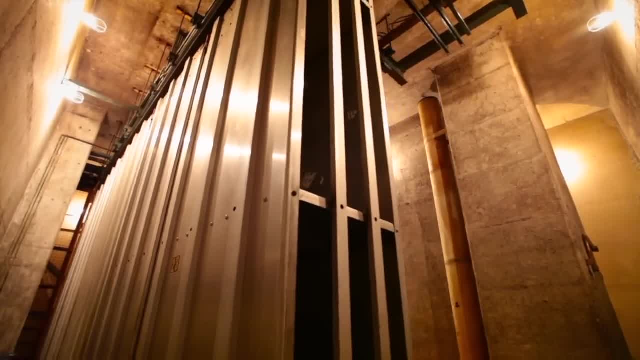 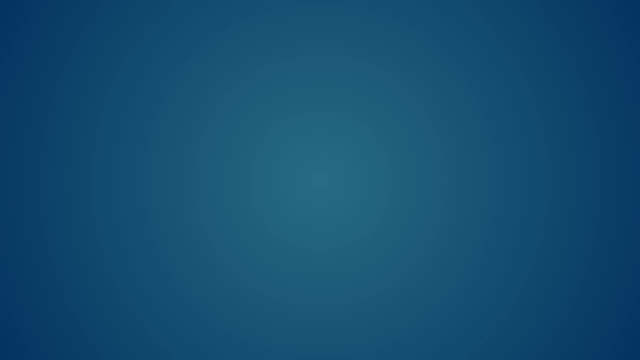 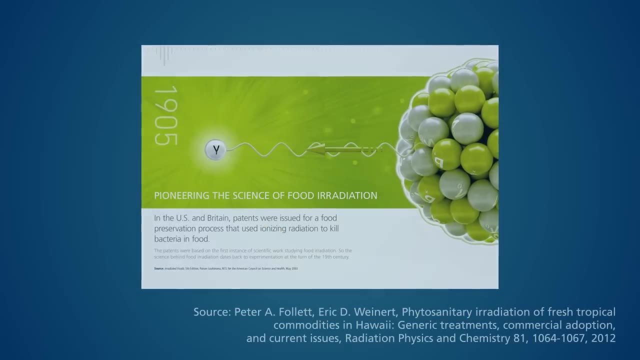 chamber. enough gamma rays pass through the spices to get a reduction in microbes and enhance the shelf life. Irradiation of food has been studied since the turn of the 20th century and used commercially for more than 50 years, With scientific data behind it. this process is endorsed by international 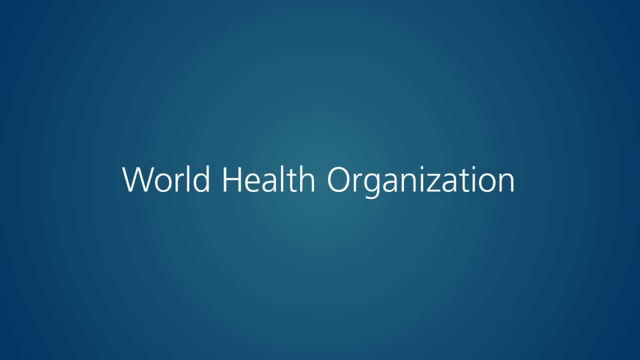 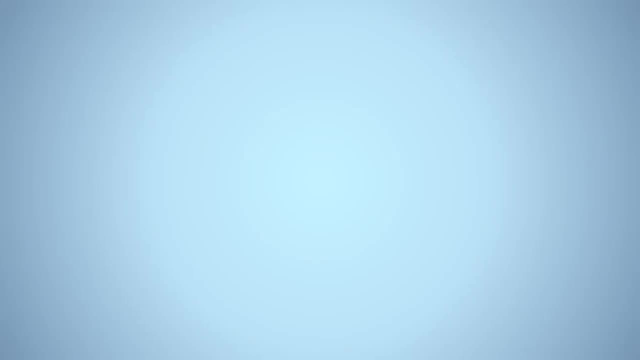 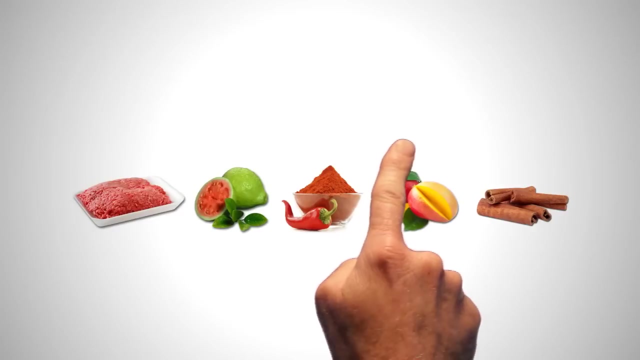 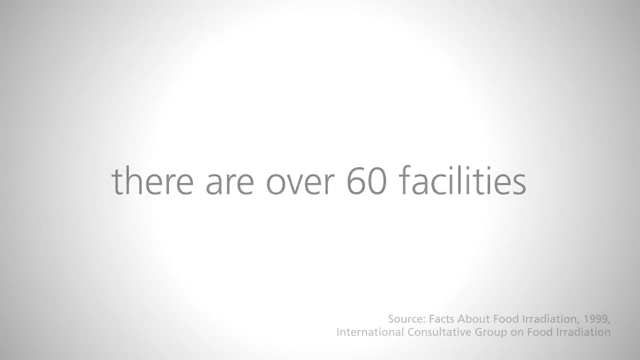 bodies such as the World Health Organization, the Food and Agriculture Organization and the American Medical Association. Retailers like Wegmans and Omaha Steaks are stocking irradiated products to meet the demand of their customers. There are over 60 facilities around the world that irradiate food products. You can work.